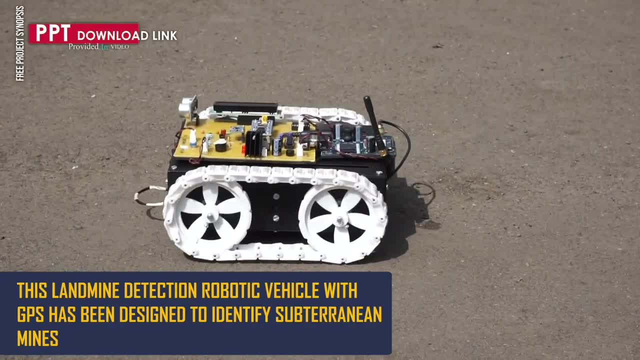 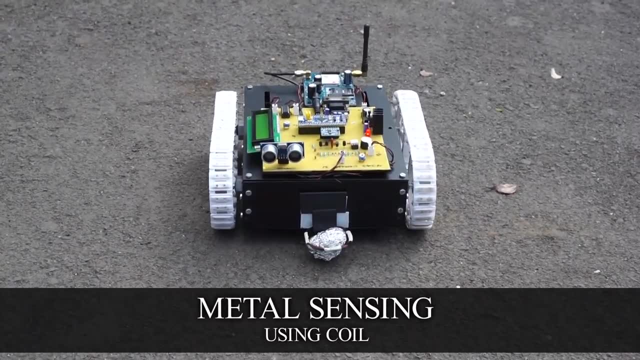 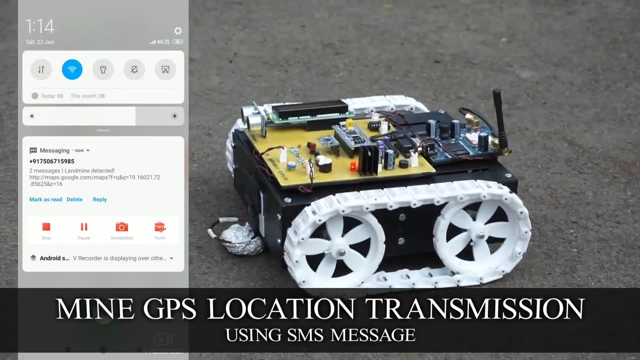 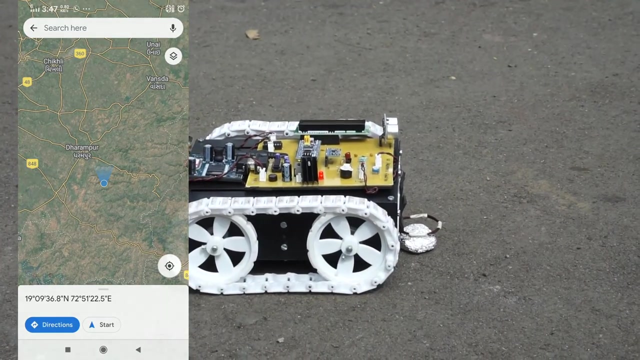 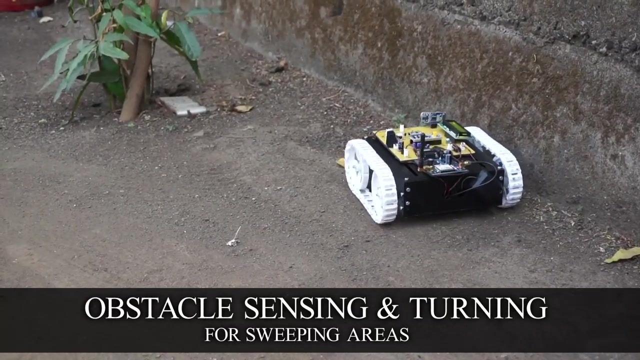 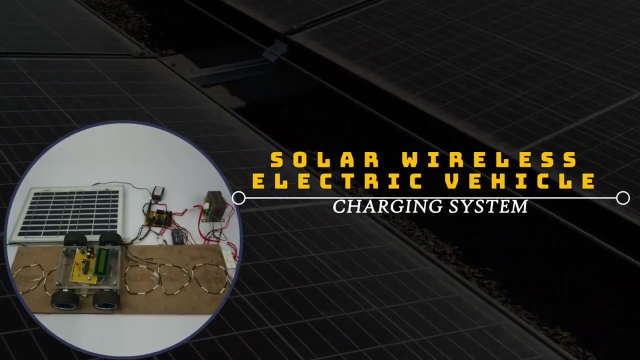 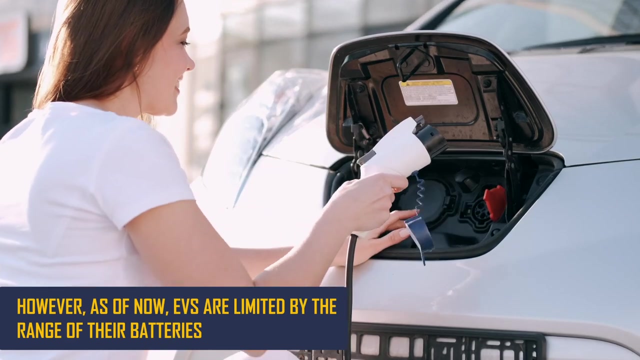 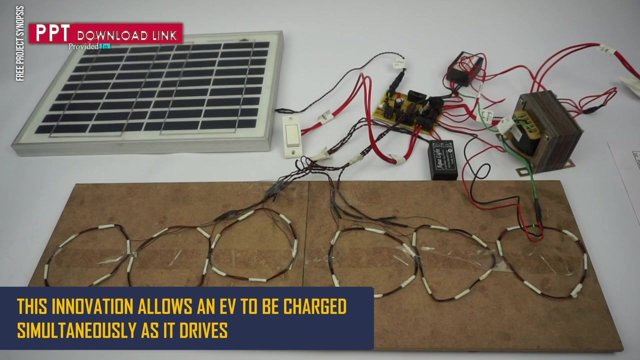 This landline detection robotic vehicle with GPS has been designed to identify subterranean mines. The solar wireless electric vehicle charging system. Electric vehicles are undoubtedly the future of transportation. However, as of now, EVs are limited by the range of their batteries. This innovation allows an electric vehicle to be charged simultaneously. 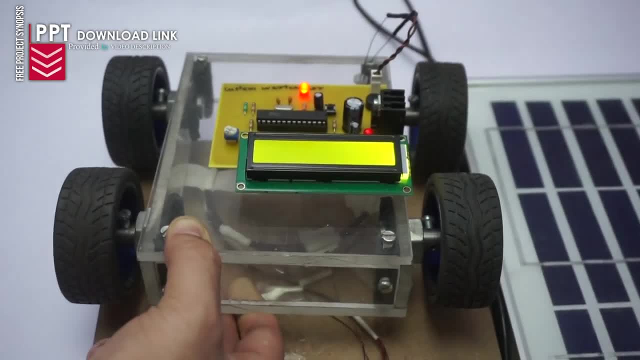 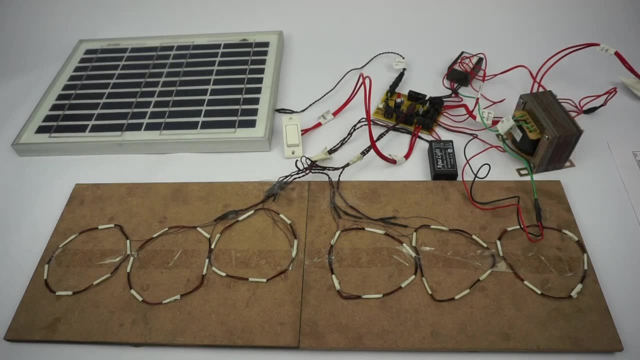 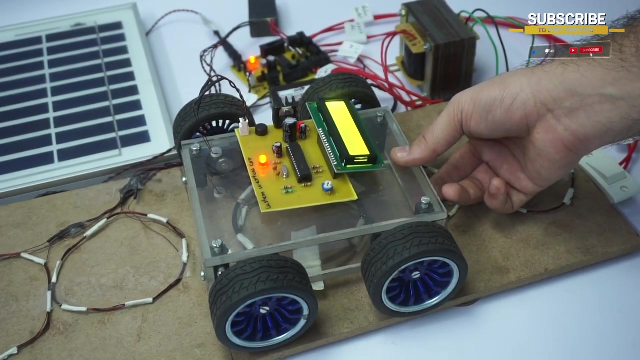 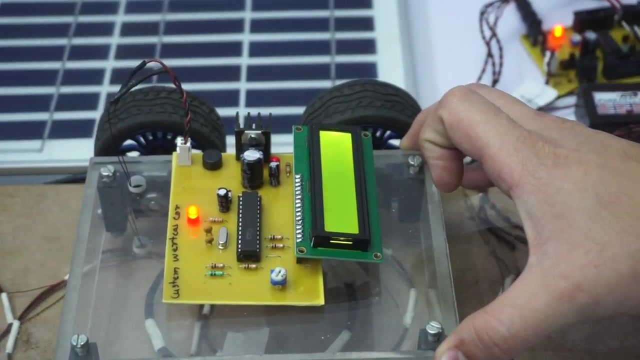 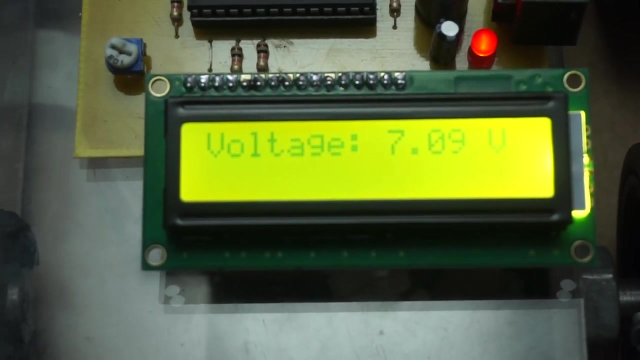 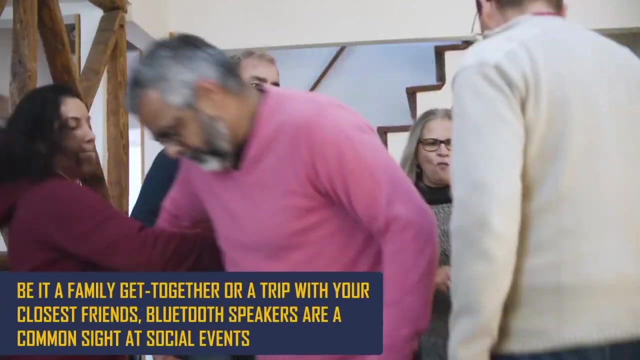 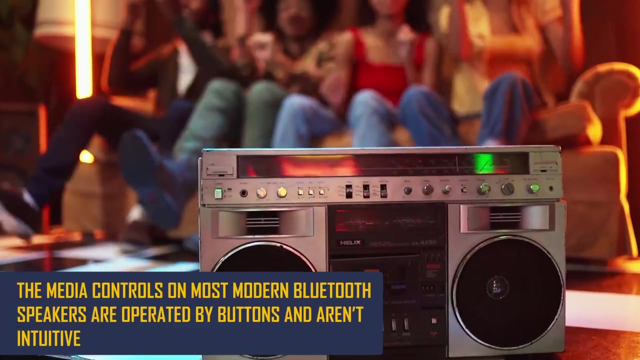 as it drives Gesture-controlled Bluetooth speaker. Be it a family get-together or a trip with your cool family, you can use this Bluetooth speaker to communicate with your closest friends. Bluetooth speakers are a common sight at social events. The media controls on most modern Bluetooth speakers are operated by buttons and aren't. 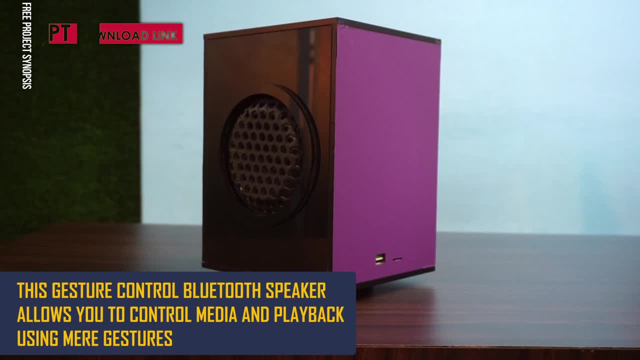 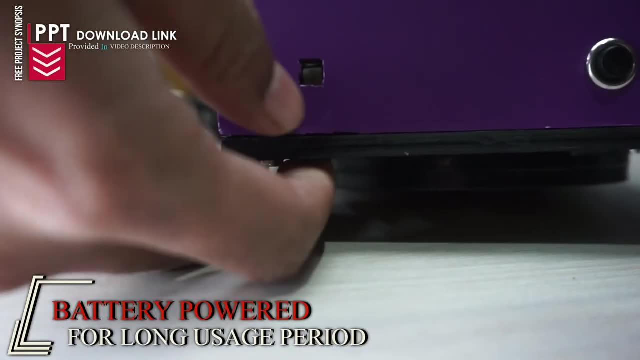 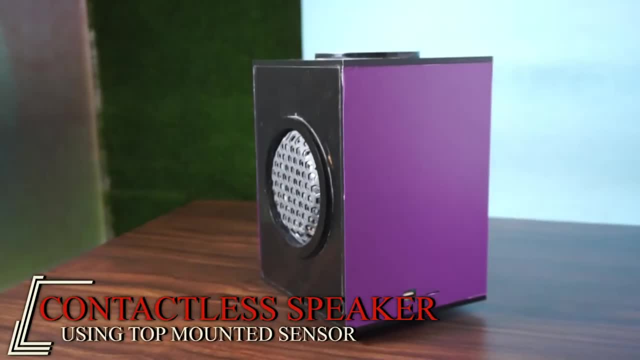 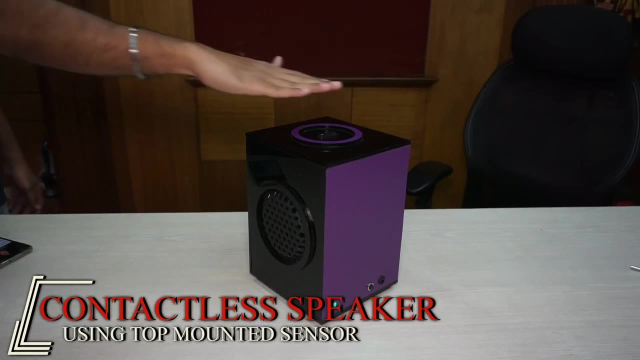 or play music, or play music to music. This Jesús-type Bluetooth speaker provides a great variety of performance. You can play music and play music through Bluetooth. If you want to do it on your own, you can enjoy playing music. Battery life of this Bluetooth speaker can be reduced to 99% with the Bluetooth app. 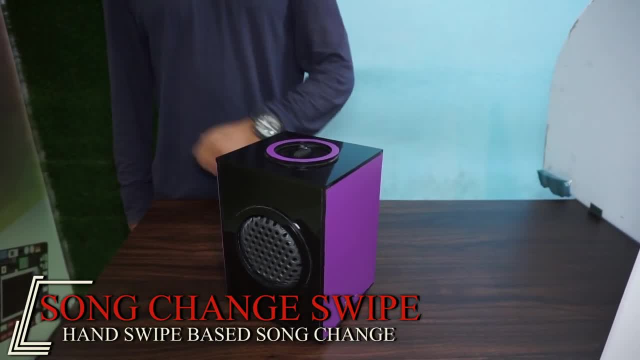 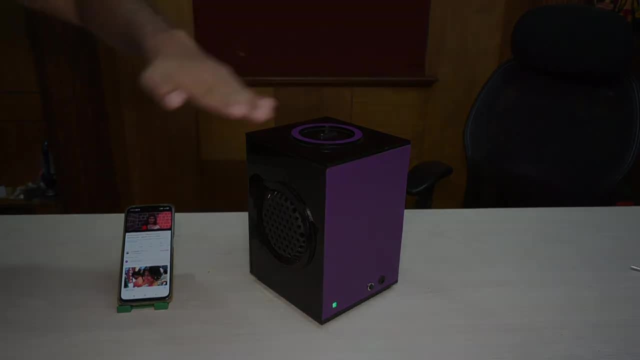 It can be used to play music, and play music with other devices. There are many other features, but this one you should never miss. Here's another video for you to check out. You can also do it with the Bluetooth app. DIY, low-cost ventilator Ventilators have been in the limelight in the 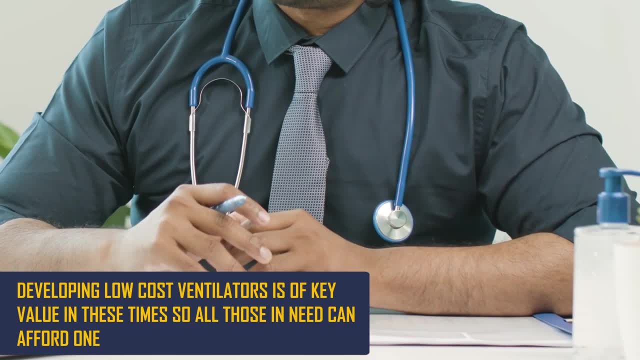 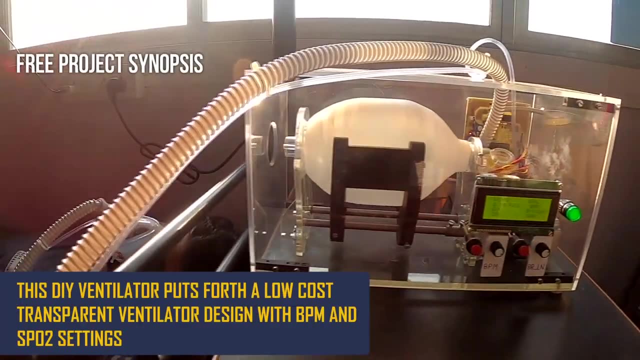 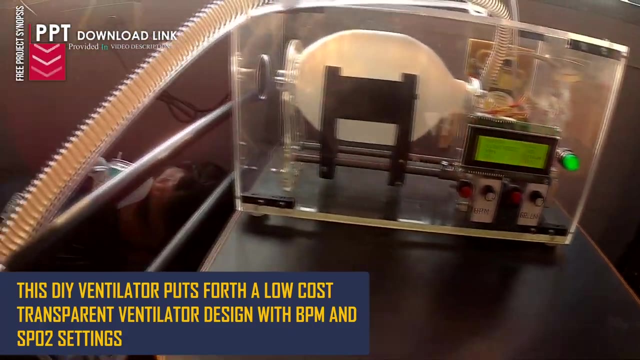 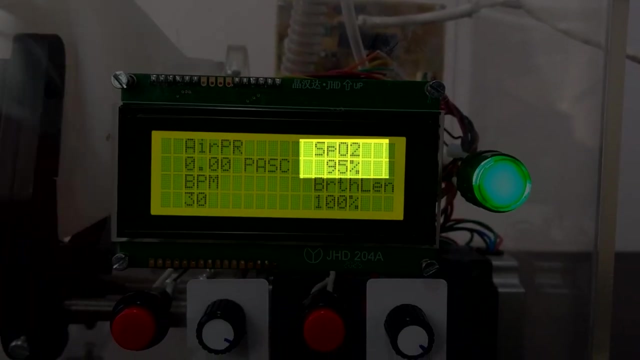 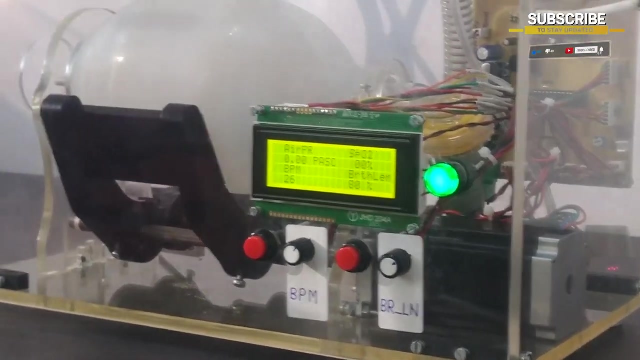 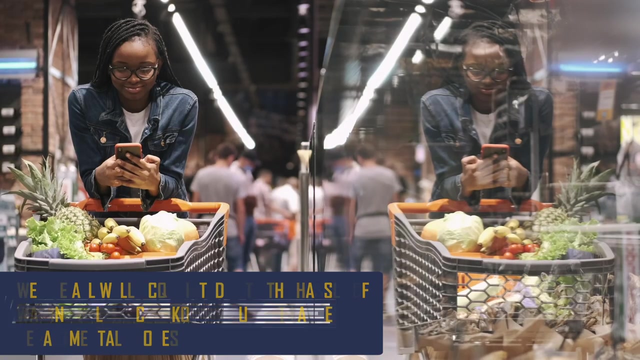 COVID crisis. Developing low-cost ventilators is of key value in these times, so that all those in need can afford one. This DIY ventilator puts forth a low-cost, transparent ventilator design with BPM and SPO2 settings. Auto Billing, Shopping Trolley using Arduino. We are all well acquainted with the hassle. 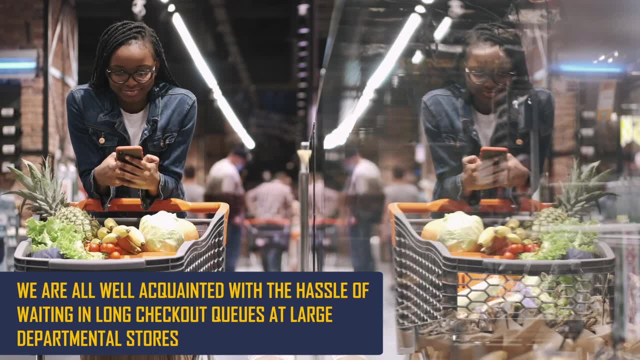 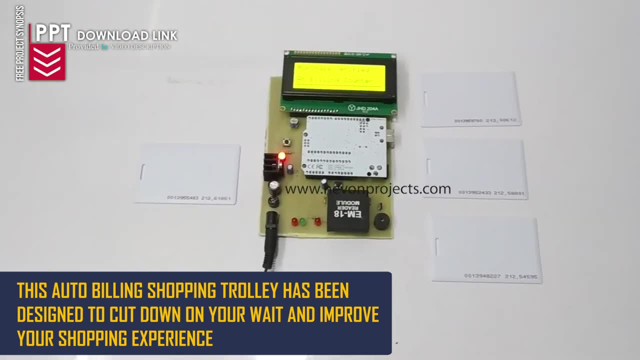 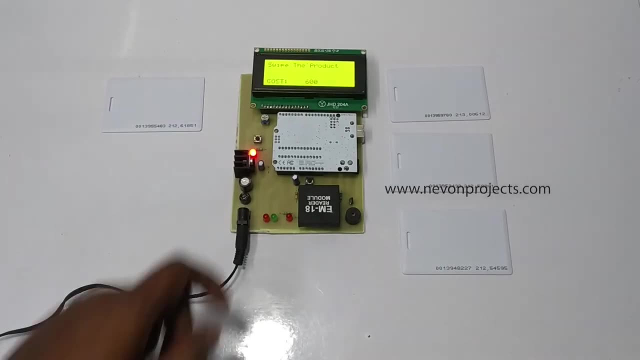 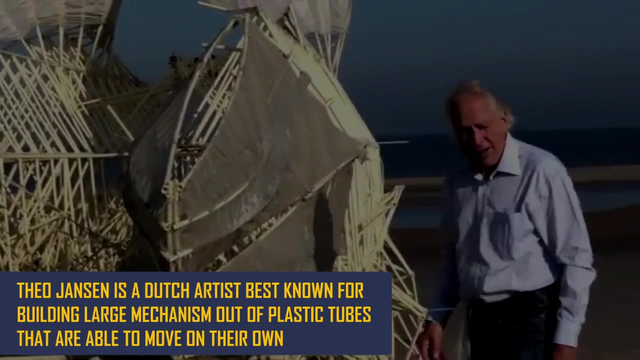 of waiting in long checkout queues at large departmental stores. This auto-billing shopping trolley has been designed to cut down on your wait time and improve your shopping experience. 8-Leg Spider Robot using Theo Jensen. Theo Jensen is a Dutch artist best known for. 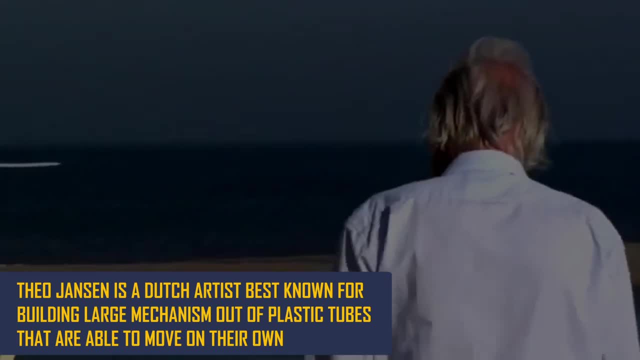 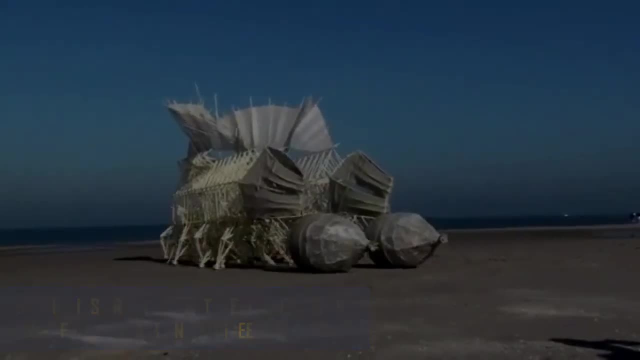 building large mechanisms out of plastic tubes. The machine is designed to be able to move on its own. Heavily inspired from nature, these machines are a fusion of art and engineering. These machines mimic the movement of animals, thus making them more efficient compared to. 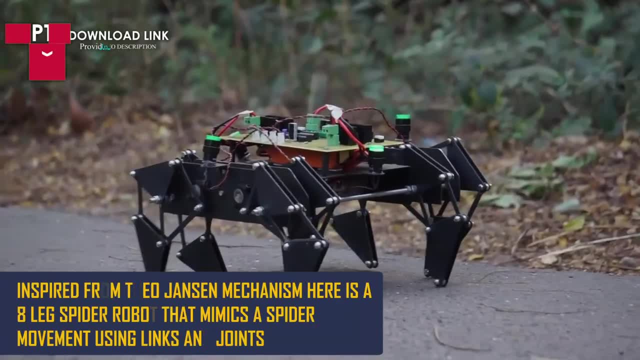 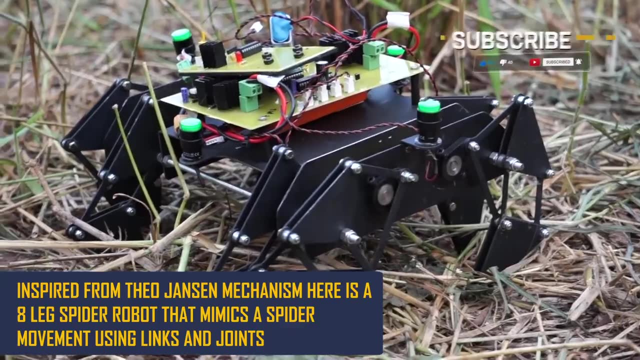 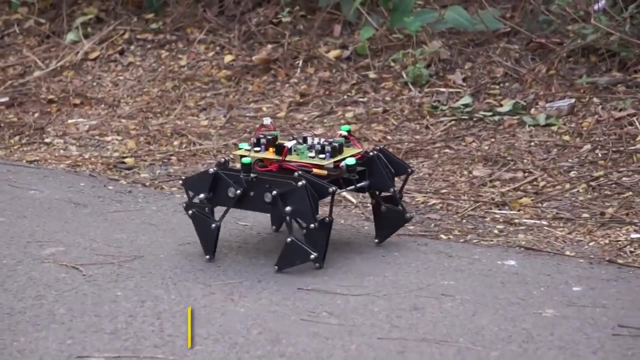 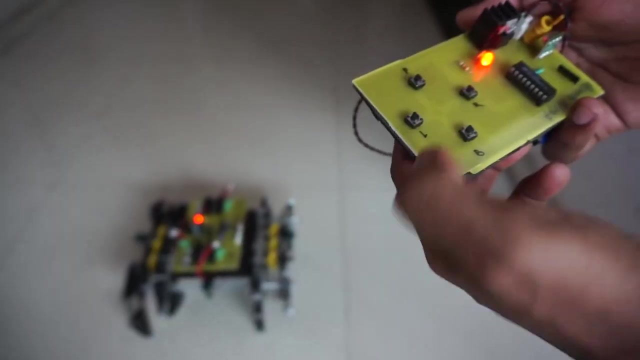 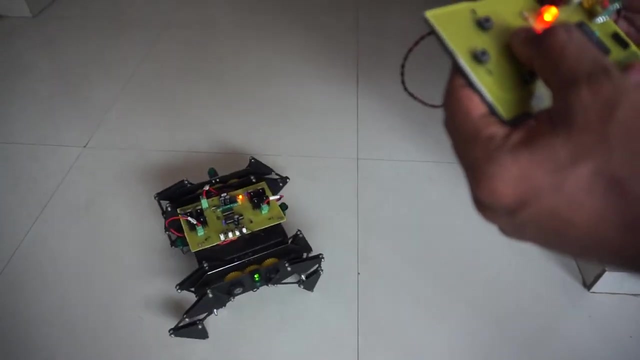 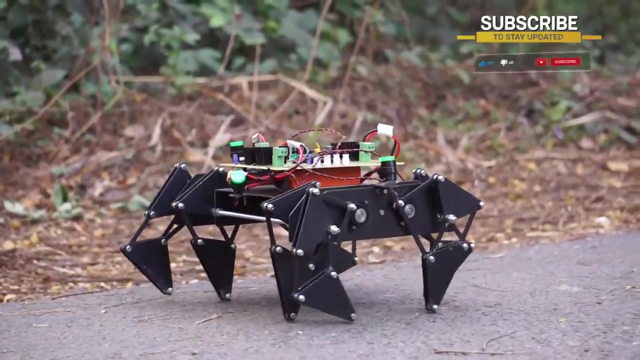 wheels over sand and rough terrain. Inspired from the Theo Jensen mechanism, this is an 8-leg spider robot that mimics the spider movement using just links and joints. These machines are made of steel and their movements are합니다 out of plastic. These machines play a vital role iniz sale. 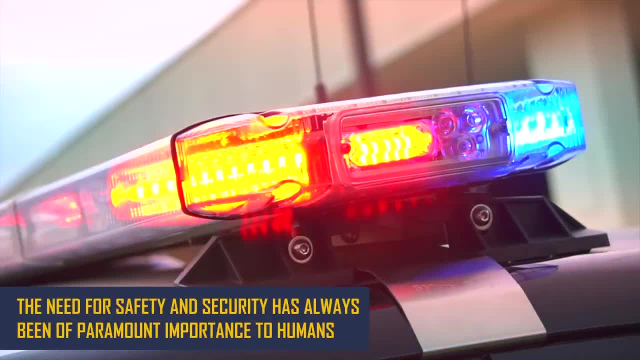 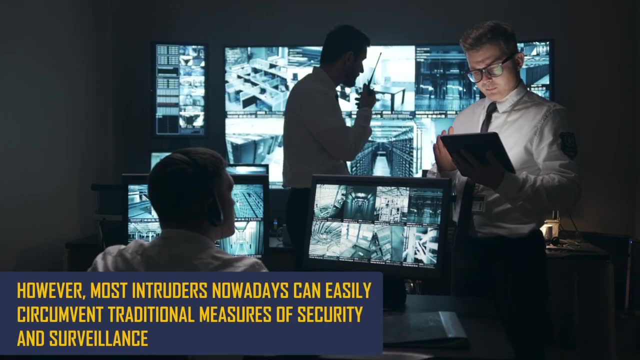 IOT- Anti-theft flooring. IOT is the name of the brand that did this. The need for safety and security has always been of paramount importance to humans. However, most intruders nowadays can easily circumvent traditional measures of security and surveillance. 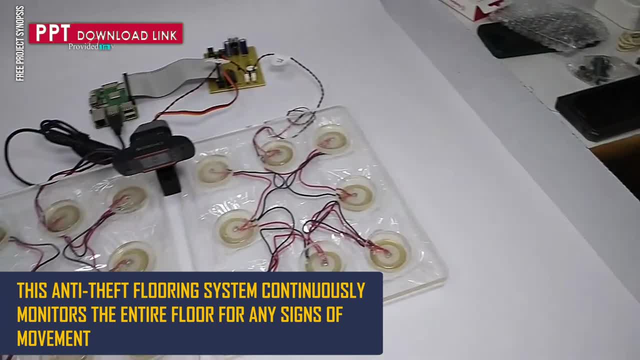 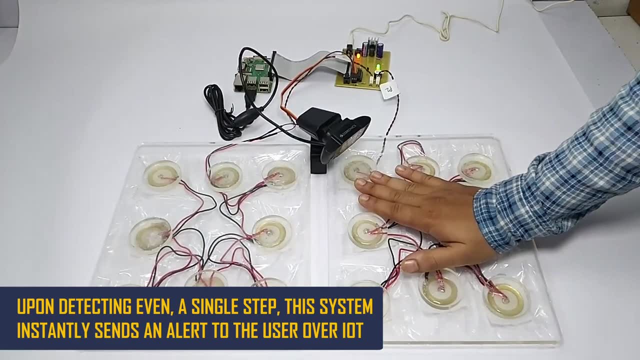 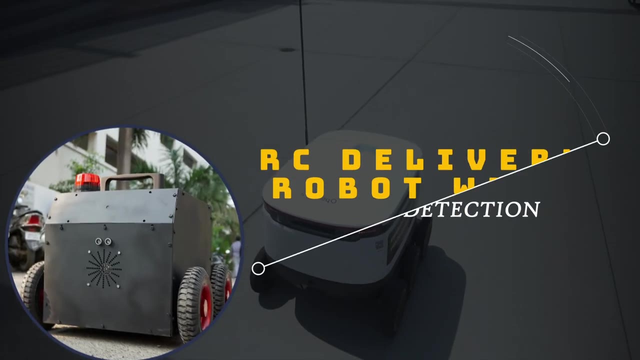 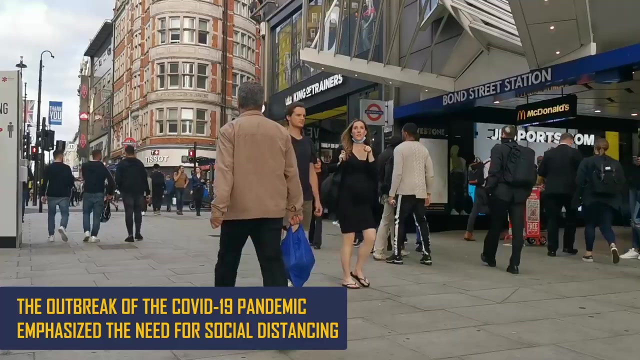 This anti-theft flooring system continuously monitors the entire floor for any signs of movement. Upon detecting even a single step, this system instantly sends off an alert to the user over IoT. 3. RC Delivery Robot with Tap Detection. The outbreak of the COVID-19 pandemic emphasized the need for social distancing. 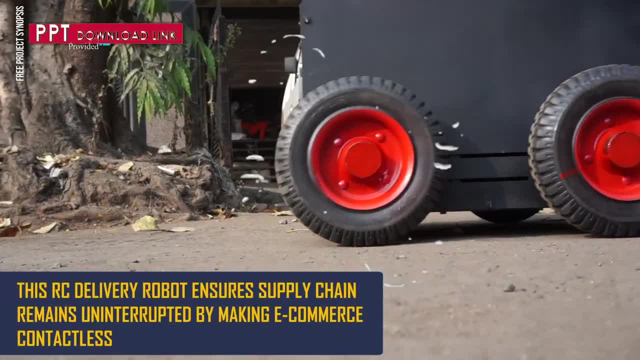 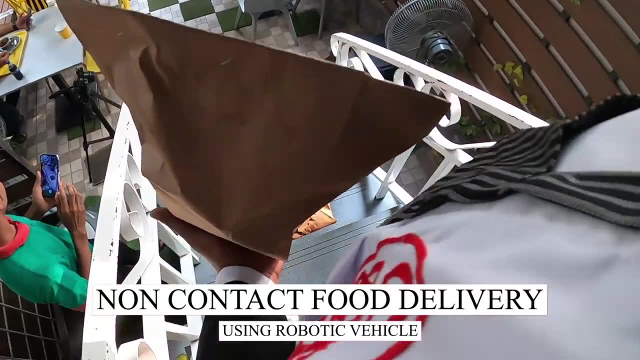 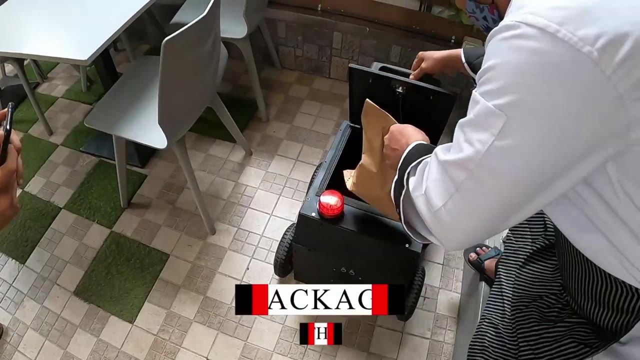 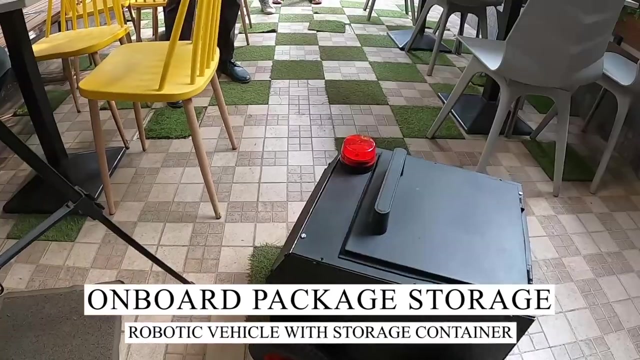 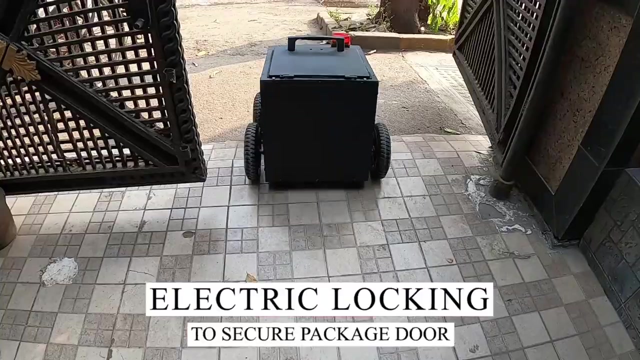 This RC delivery robot ensures supply chain remains uninterrupted. by making e-commerce contactless, Thisител24 provides a level of security for the user, at least as far as it goes. 4. Downtown, The Recruitment Area, is home to the most modern city in the country. 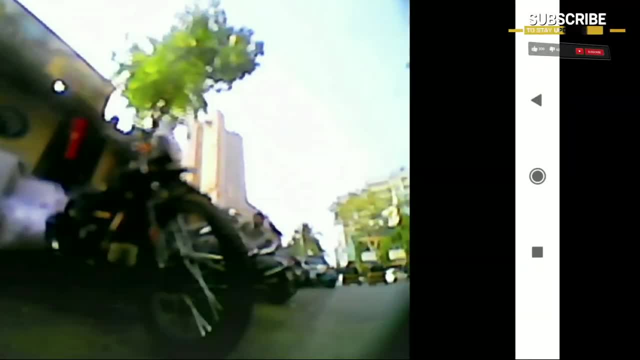 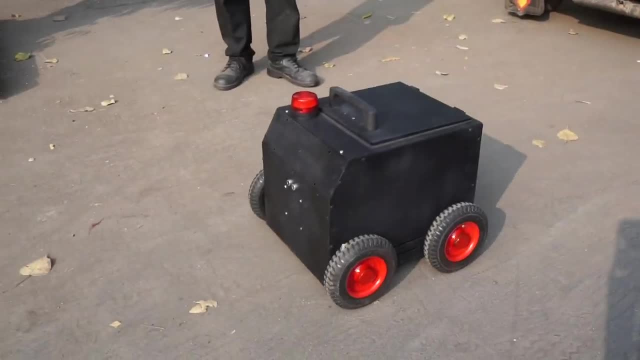 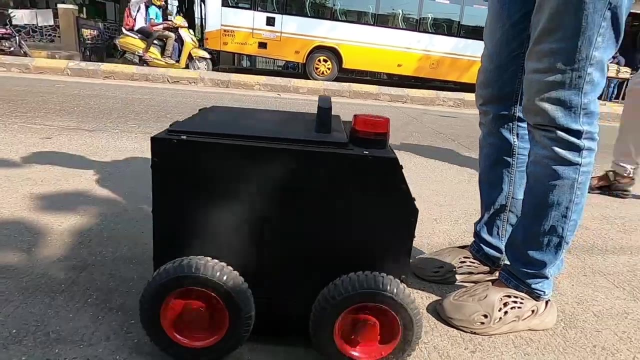 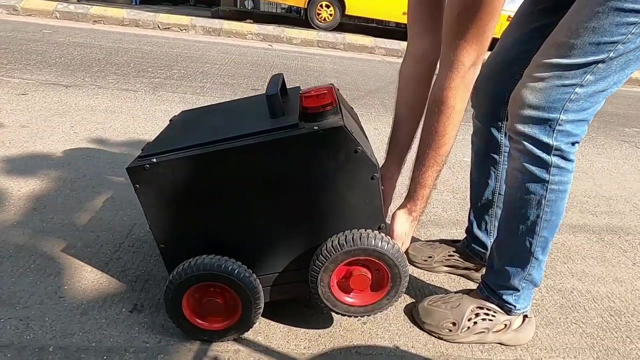 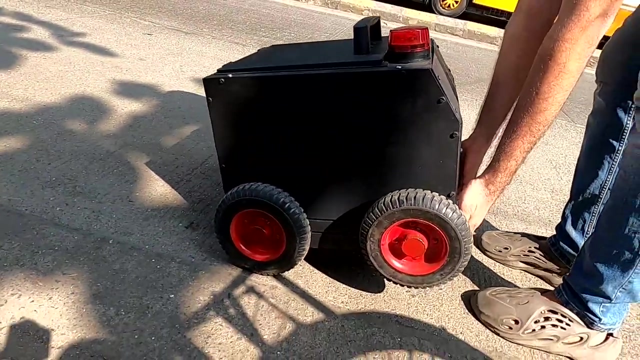 This feature includes a large area with about 3,000 people attending the event. This is a great lakefront area and it is one of the most modern tourist destinations in the United States. 5. Ferry Park Smart Energy Meter Monitor with Tap Detection. 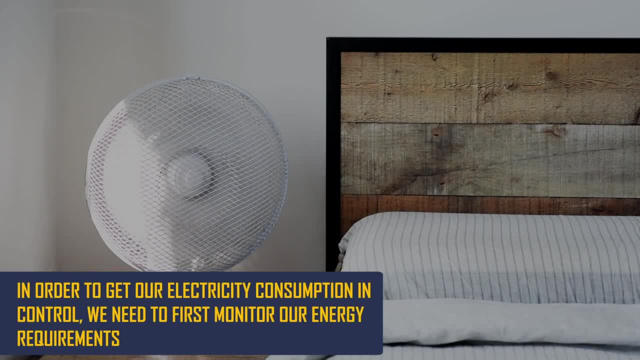 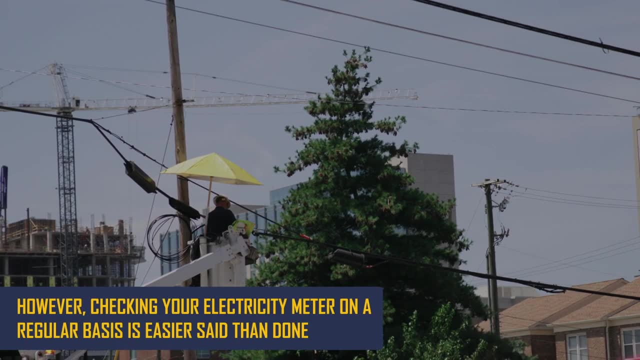 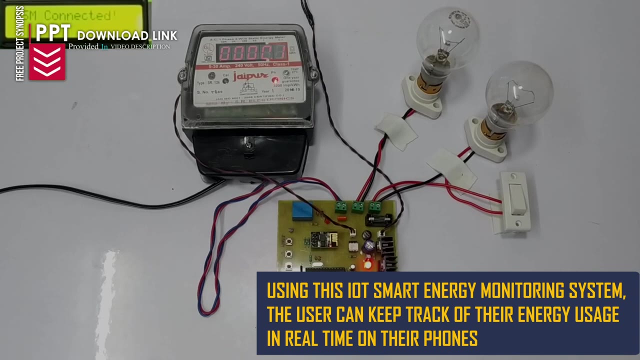 In order to get our electricity consumption in control, we need to first monitor our energy requirements. However, checking your electricity meter on a regular basis is easier said than done. Using this IoT smart energy monitoring system, the user can keep track of their energy usage. 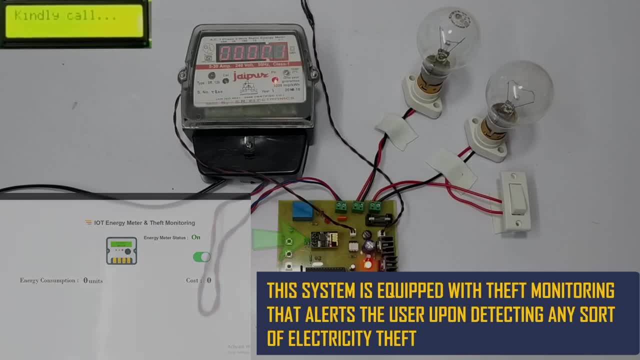 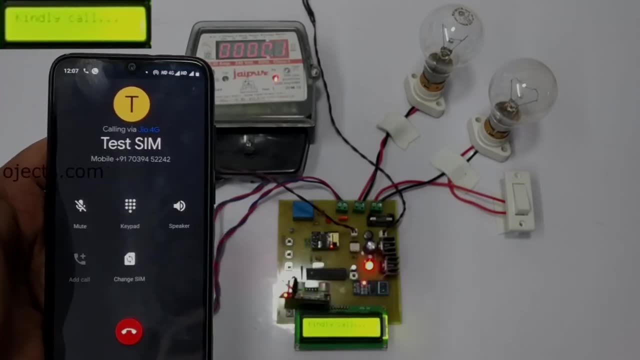 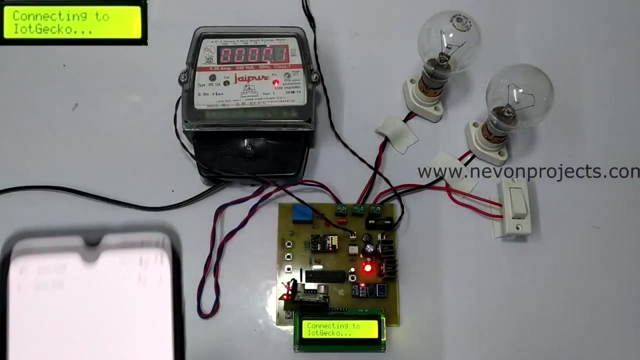 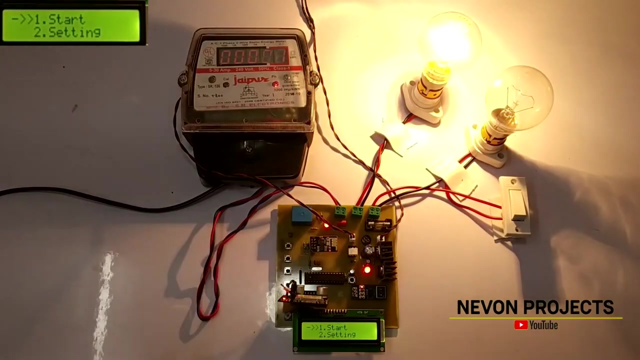 in real time on their phones. The system is equipped with theft monitoring that alerts the user upon detecting any sort of electricity theft. With its advanced IT technology, the user can easily monitor and track the latitude of the electricity that is being used in the environment. 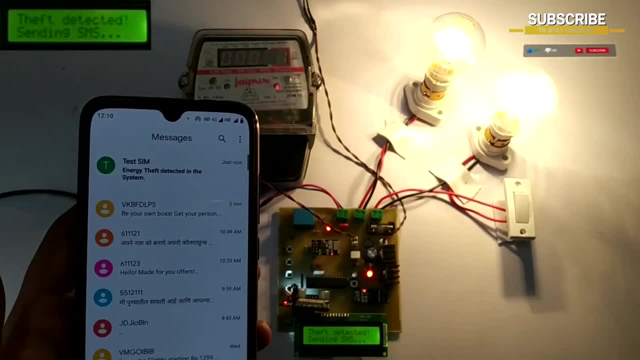 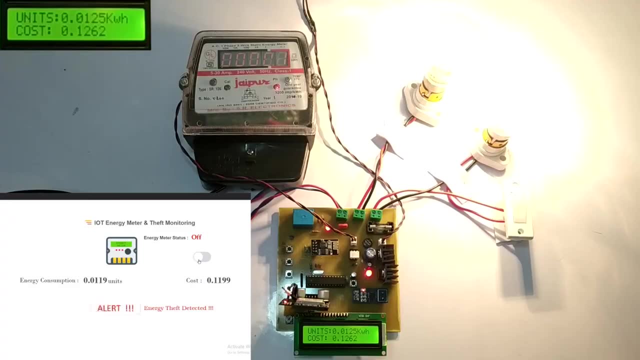 The IoT smart energy monitoring system also lets you monitor theות, current electricity levels and temperature. This is the equivalent of 60°C. If we set the energy level in a small mode, the IT will simply monitor the temperature and temperature of the electricity. The IoT smart energy monitoring system will notify the Elixir temperature meter and switch on and off the power button. If we switch off the power button, the IoT smart energy monitoring system will notify the Elixir temperature meter and switch on and off the power button. 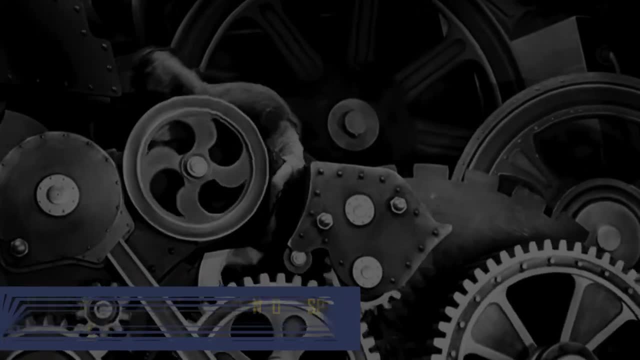 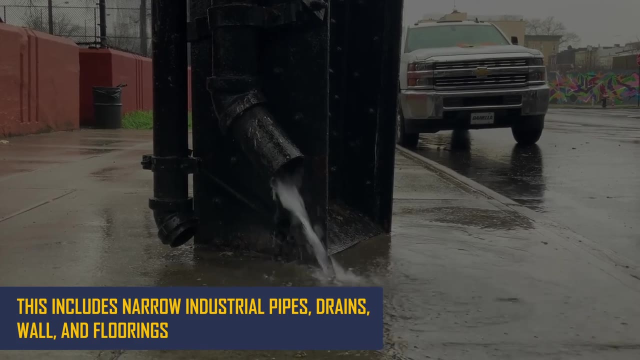 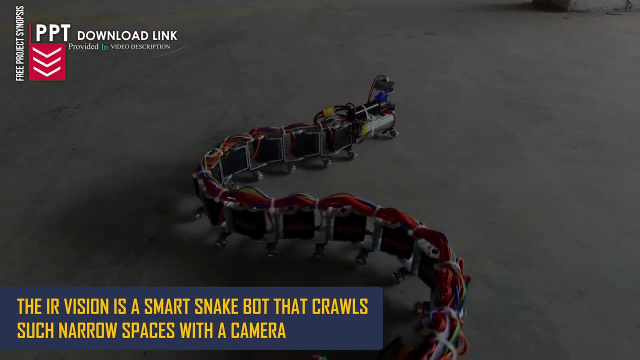 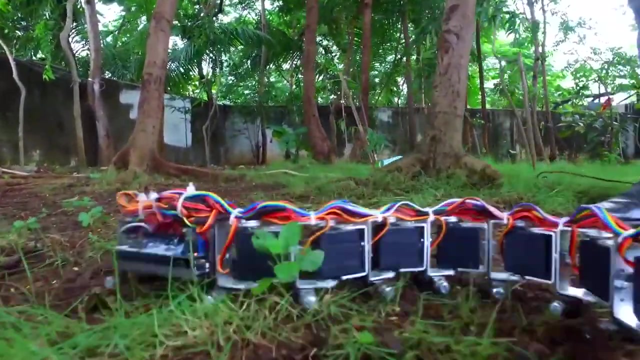 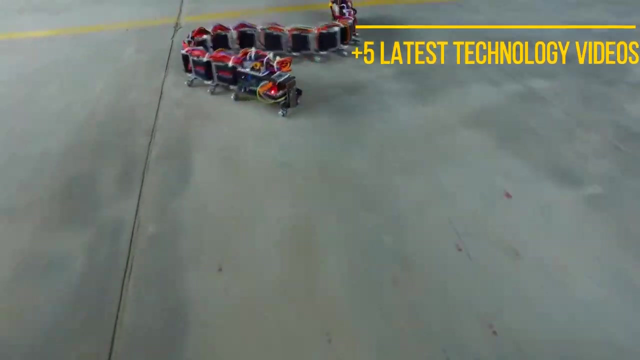 based snake robot for inspection. Humans and four-wheel robots cannot inspect tight spaces. This includes narrow industrial pipes, drains, wall and floorings. The IR Vision Snake Robot is a smart bot that crawls such narrow spaces with a camera. Introducing LR Robot. 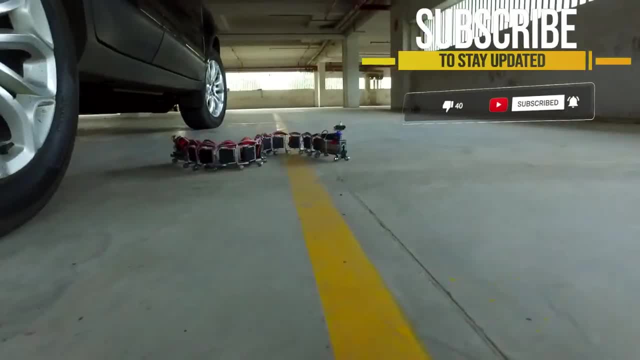 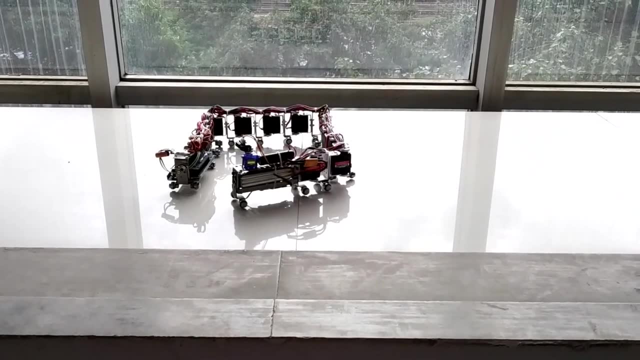 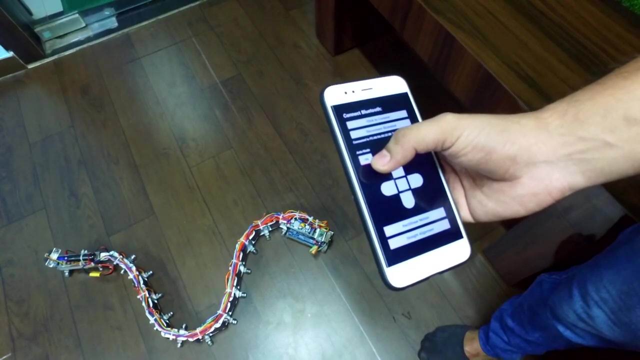 The LR Robot is an artificial intelligence robot built in CSF Technology ISE. The LR Robot is a smart robot that's used to inspect the center of theumpair. It's a smart robot that uses its power to enter and exit theah问. 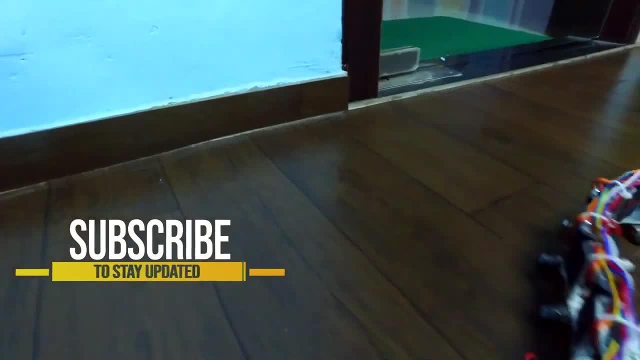 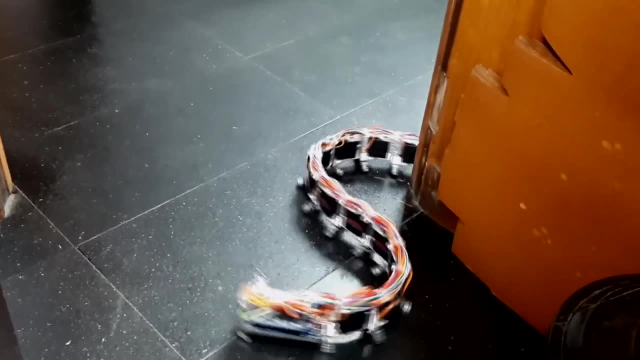 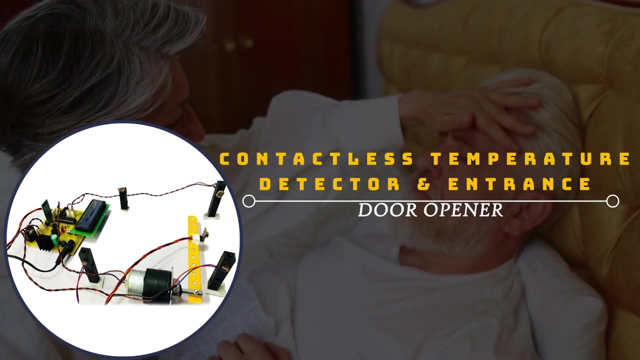 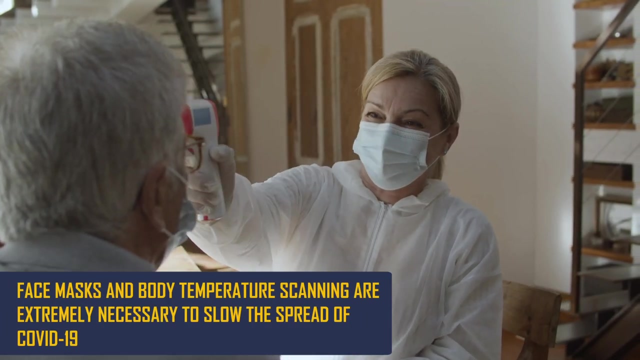 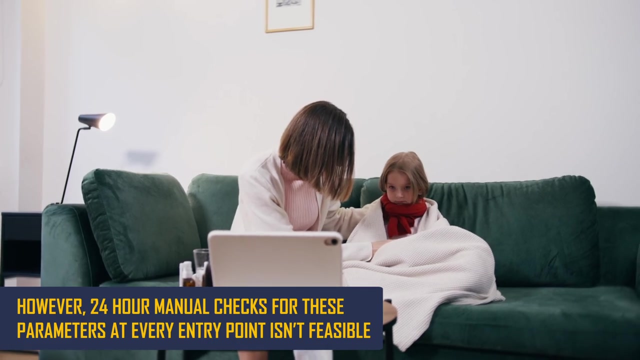 Contactless temperature detector and entrance door opener, Face mask and body temperature scanning are extremely necessary to slow the spread of COVID-19.. However, 24-hour manual checks for these parameters at every point isn't feasible. This contactless temperature detector and entrance door opener automates the monitoring. 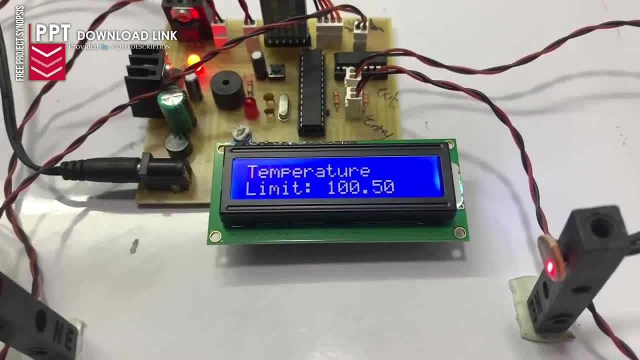 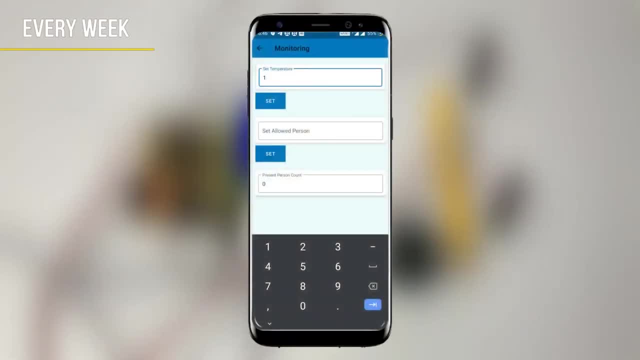 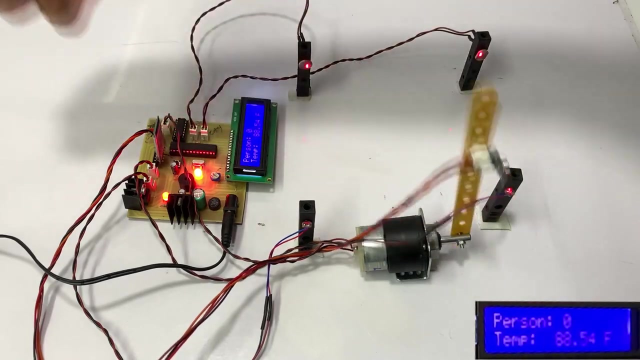 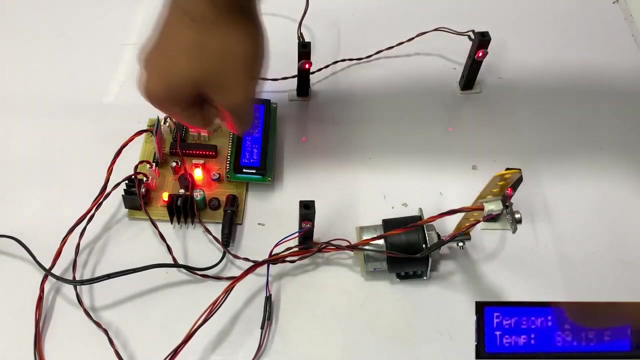 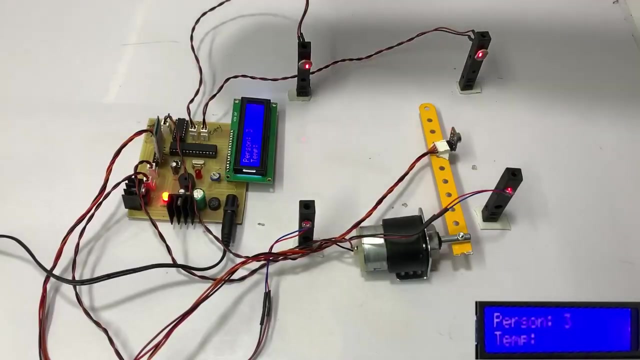 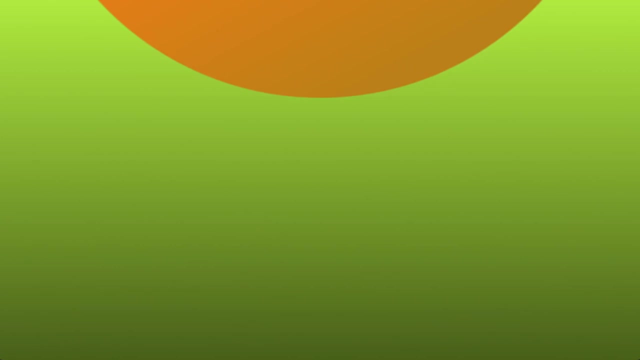 of masks, as well as scanning for temperature. If you have any questions or other problems, please post them in the comments section below. Thank you for watching and have a great day. Bye, Bye, Bye.